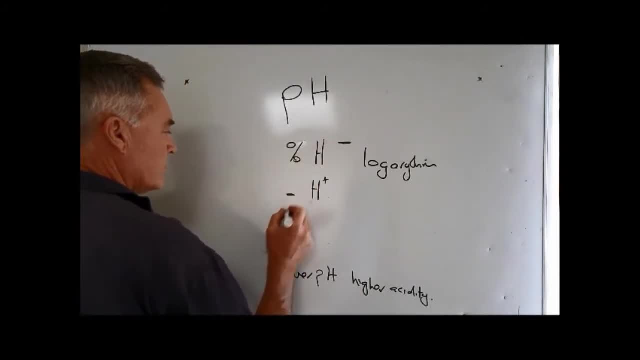 easily exchangeable. Every negative site in the soil will be filled with a hydrogen as long as there are no other cations. So if there's no calcium, magnesium, potassium or sodium, hydrogen will go onto the site. When that happens, the more hydrogen there is. 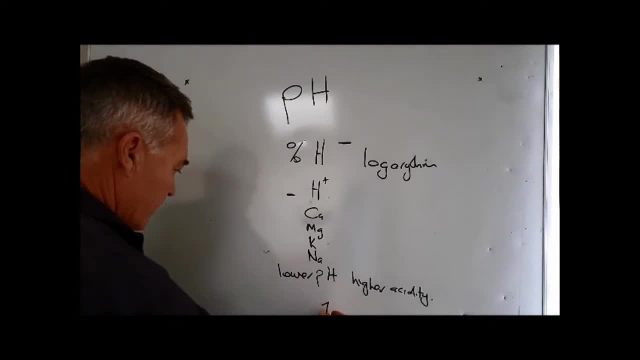 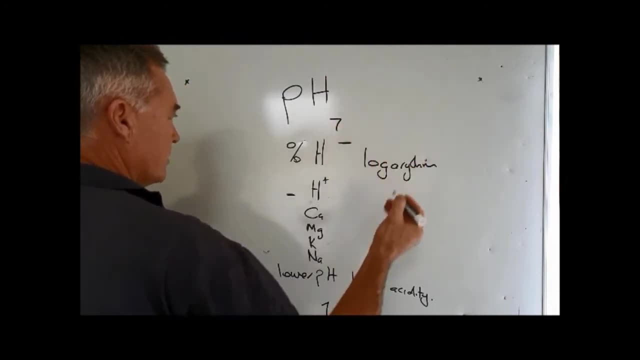 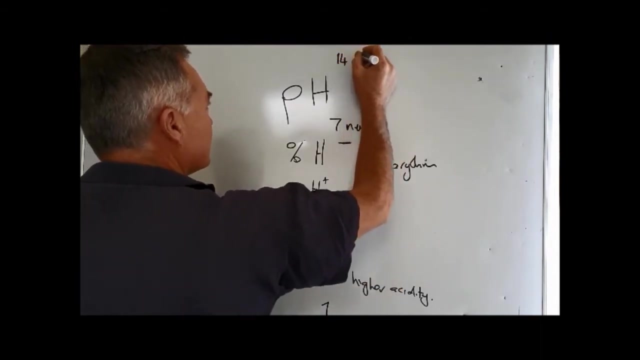 the lower the pH, And we start at a scale of 1, and we go to 7,, being- what do you call it? neutral, And then you go to an alkaline of up to 14.. So what's happening in the soil is you will. 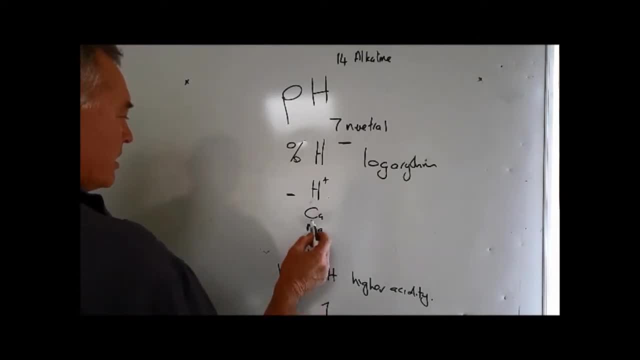 change the pH by changing the cations. So when you look at the soil sample, you need to use the cations more than you look at the hydrogen. It's great The pH is utilised. when you measure the parts per million of these minerals against the pH, Use that as a calculation. 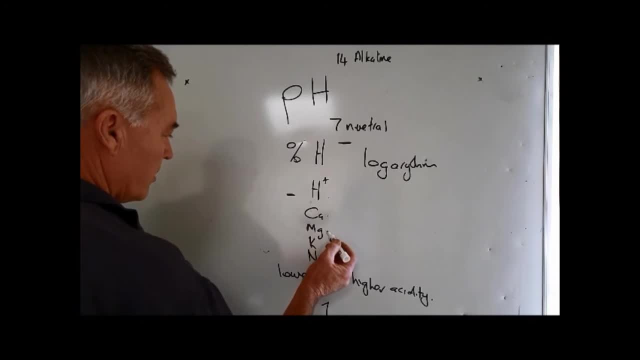 Then it will tell you the percentage of how much of these minerals are in the soil And then you can work out how much you need to apply to increase the pH. But always remember pH is a result, not something you should gauge. what you should do next, Because if you look at magnesium on high magnesium soils the ph might be 6.5 up. i've seen it up to 8 in the states. and yet if that isn't completely out of balance with the magnesium, that might have a very high ph and you would decide not to apply anything. yet it may respond incredibly well. 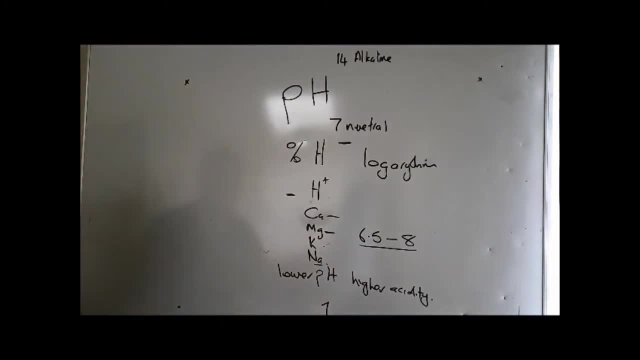 from calcium to get the balance right now. we'll go into those equations later, but this is the reason why we don't want to look at ph as a driver of decisions on how we go about making our fertilizer applications. it's very, very dangerous. so when you look at it, you look at 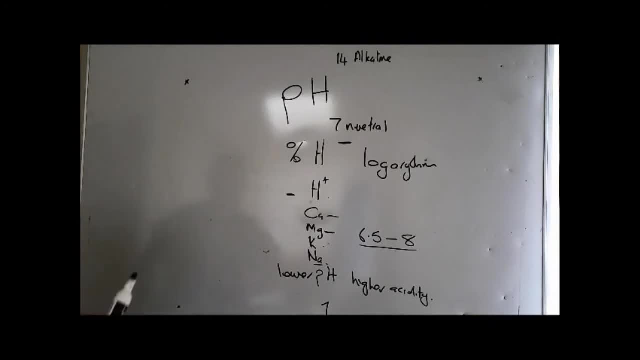 your ph test. but then go down and look at the parts per million of the major cation drivers and then look at how that can change. like i'll give you another example: if you've got really high sodium soils, you might have a ph of seven and yet